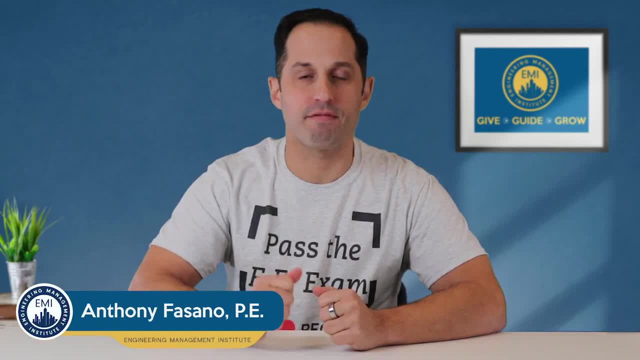 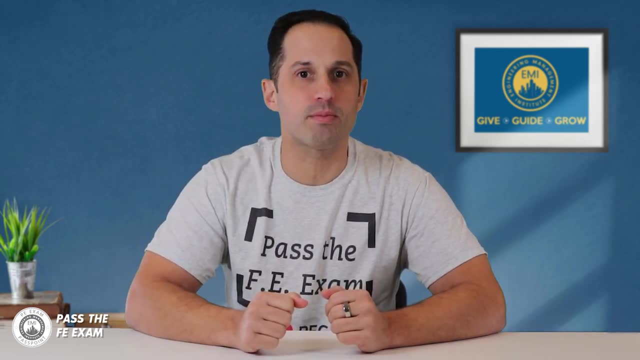 You're watching FE exam prep with Anthony Fasano from Pass the FE exam. In this video, which is the third in a five-part series about the five different civil engineering disciplines that you can choose from, we will discuss the roles, responsibilities and credentials needed to become. 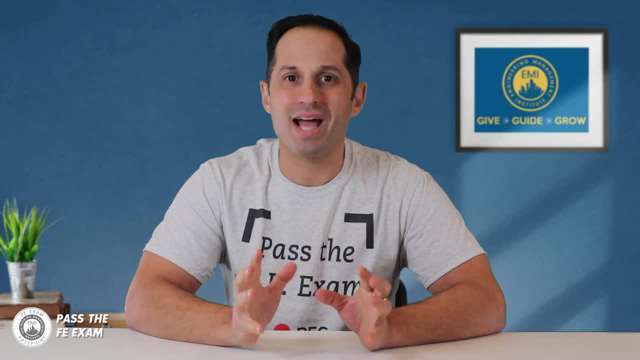 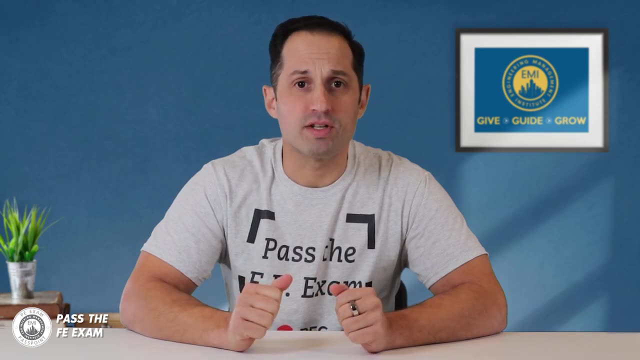 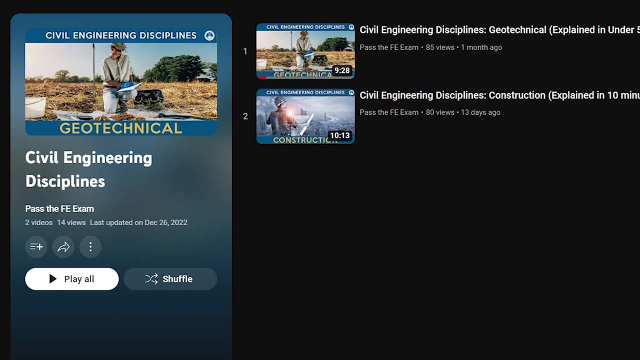 a civil structural engineer to give you a better idea of what to expect both for your studies as well as for the FE exam. In the previous videos in this series, we've discussed geotechnical as well as construction, which you can find right here on our playlist entitled. 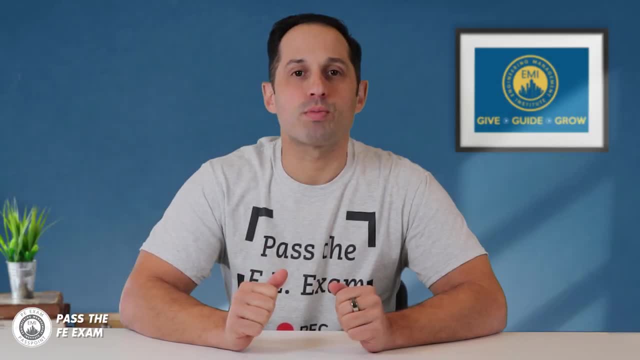 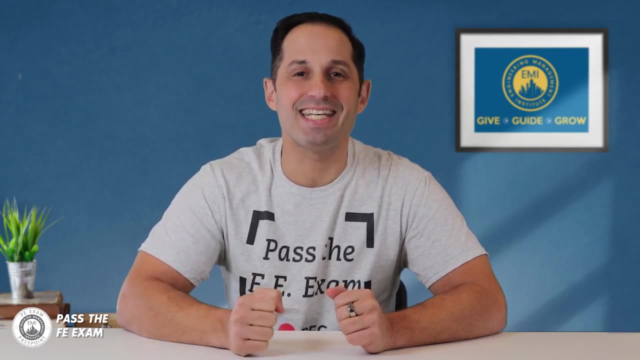 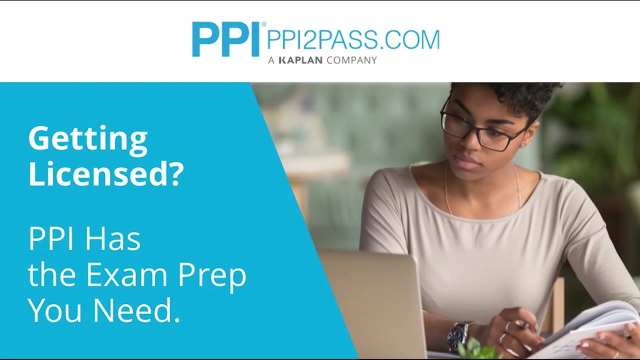 Civil Engineering Disciplines. This video is brought to you by PPI, a leader in engineering exam prep for the FE and PE exams since 1975.. PPI provides expert prep courses and study resources designed to help you pass the FE exam the first time. 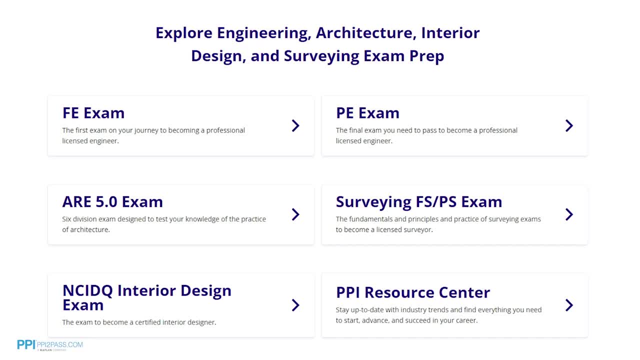 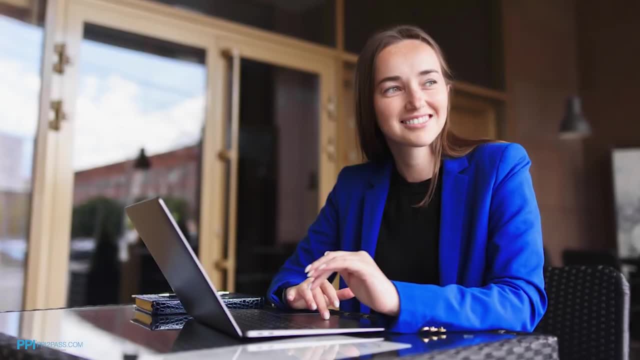 PPI's live online courses include hours of lectures, problem-solving demonstrations, exam strategy sessions, office hours and a passing guarantee. When you take a live online course, PPI guarantees you will pass, or you can take the on-demand course for free With study. 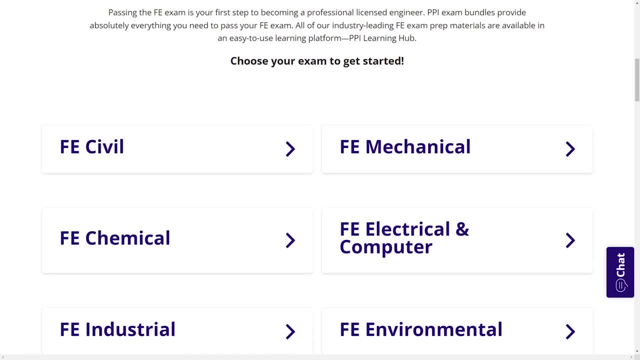 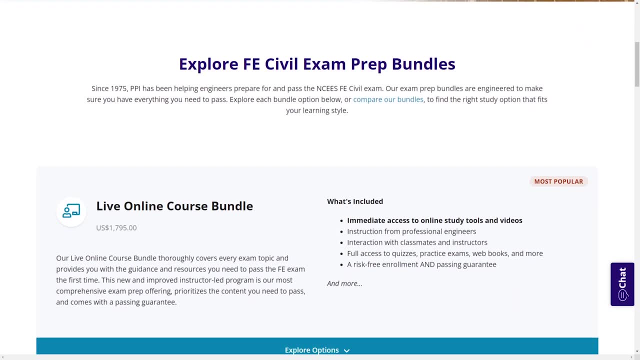 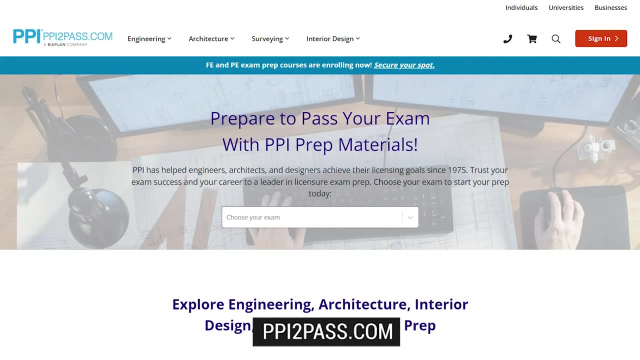 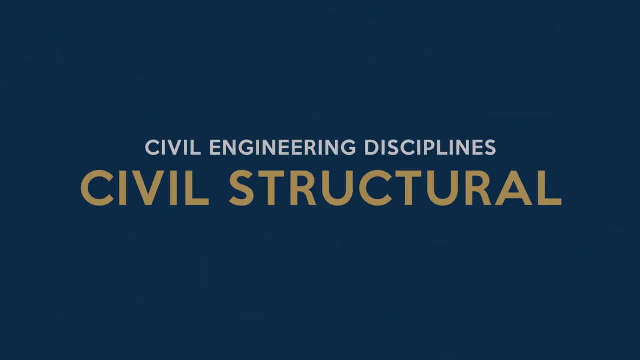 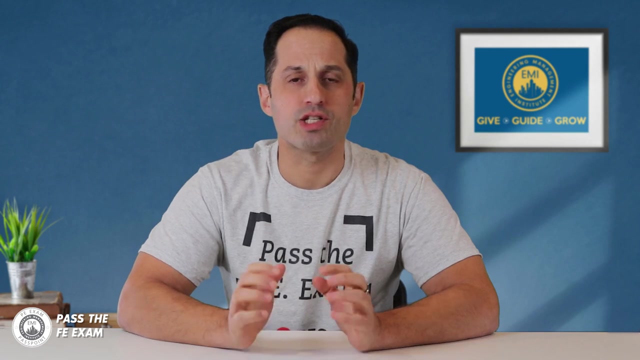 guides, practice exams and more. the PPI Learning Hub offers digital practice and review that you can take with you anywhere you have a device, so that you can prepare during the times most convenient for you. Check out PPI today. Now, before we get started, I just want to mention: 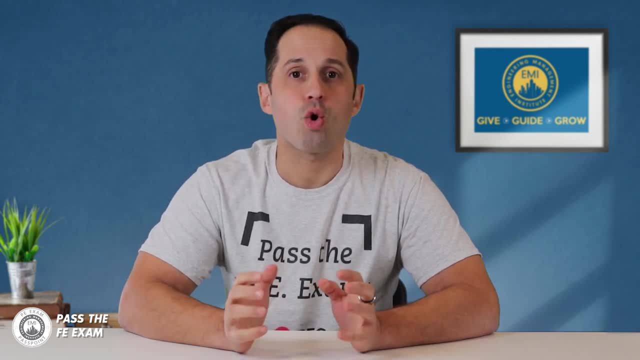 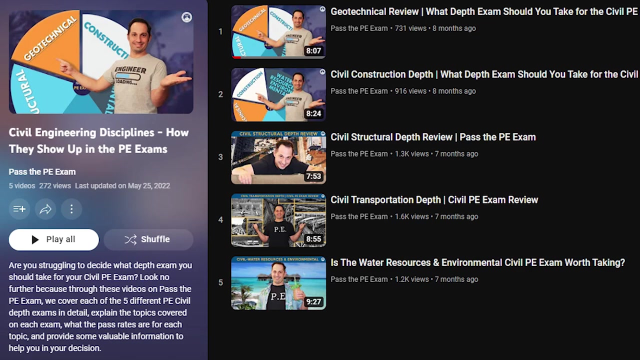 especially for those of you who already took your FE exam or are getting close to taking the exam and are thinking of taking the civil PE exam as a next step, that we did a complete series on our Pass the PE Exam YouTube channel explaining each of the five different PE civil depth exams. 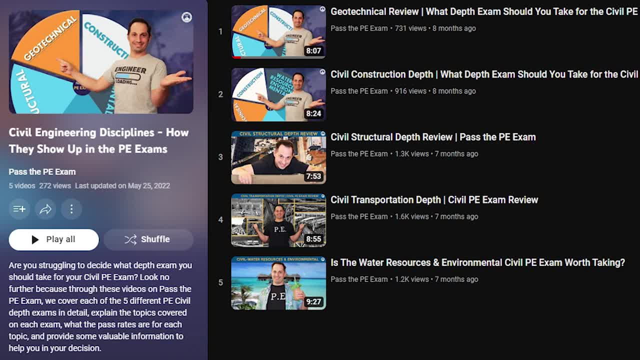 in detail, including the topics covered on each of the exams and what the passing rates are for each topic, to help you decide which one you should pursue. You can check it out on our Pass the PE Exam YouTube channel playlist at youtubecom. forward slash at Pass the PE Exam. 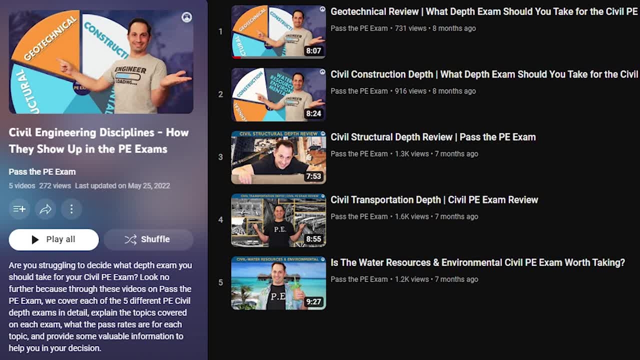 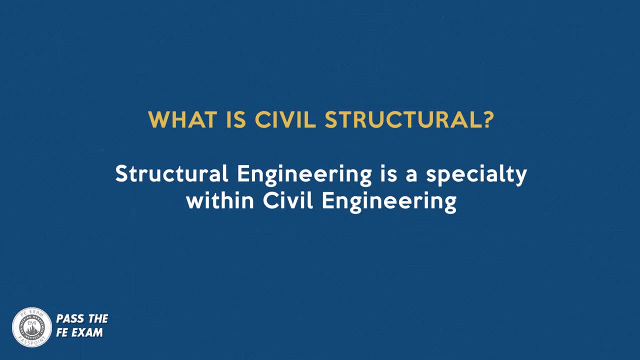 called Civil Engineering Disciplines How They Show Up in the PE Exams. Let's start by defining what a structural engineer does. Structural engineering is a specialty within civil engineering, although some say that it is a discipline all on its own And they can make a 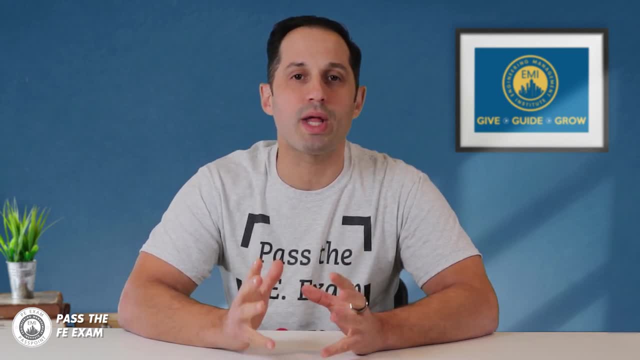 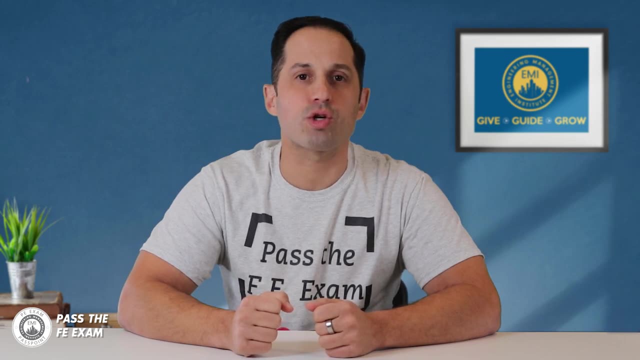 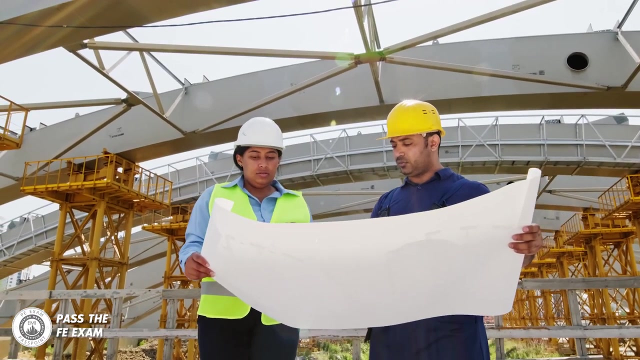 good argument for that, since there is a separate structural engineering license, typically referred to as the SE, that is required in some states. Structural engineers create drawings and specifications, they perform calculations, review the work of other engineers, write reports and evaluations- yes, you have to write- and they also observe construction. 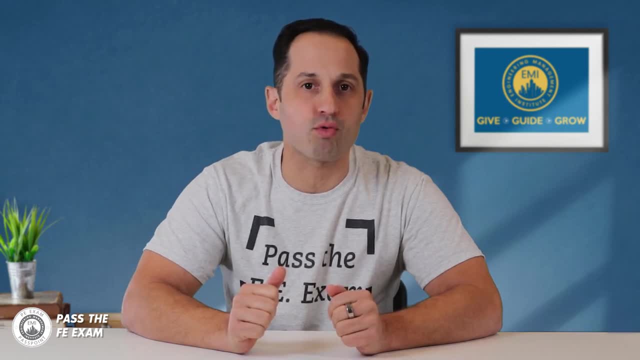 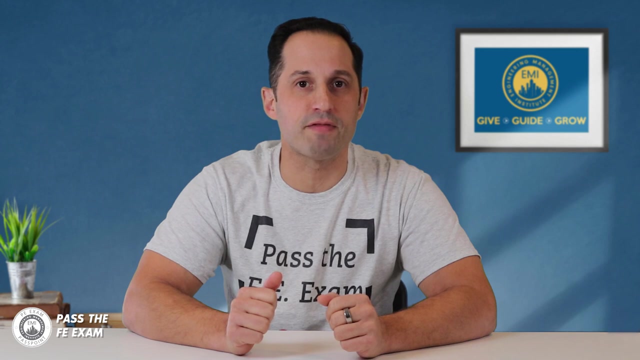 A professional engineer's license is required in order to practice structural engineering and, as I said earlier, an SE license may also be required, depending on your location of practice. The basic tasks of structural engineering relate numerical quantities of physical forces to physical configurations of force-resisting elements. 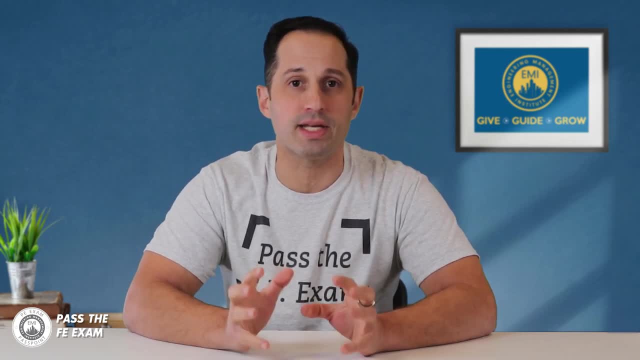 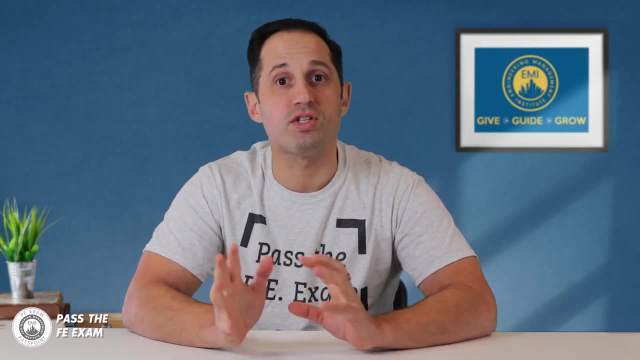 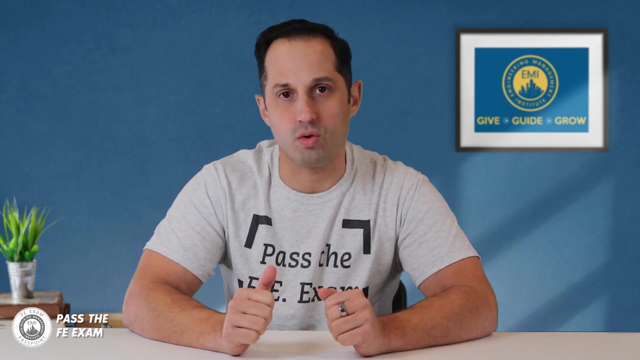 Analysis is the process of determining forces in each element in a structure such as a beam, when the configuration of the element is already defined, while design is the process of configuring elements to resist forces whose values are already known. Analysis and design are complementary procedures in the overall 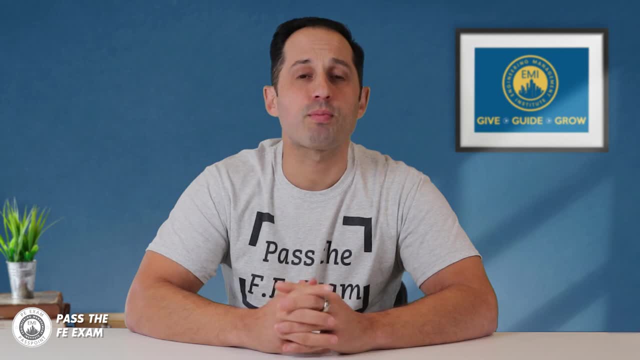 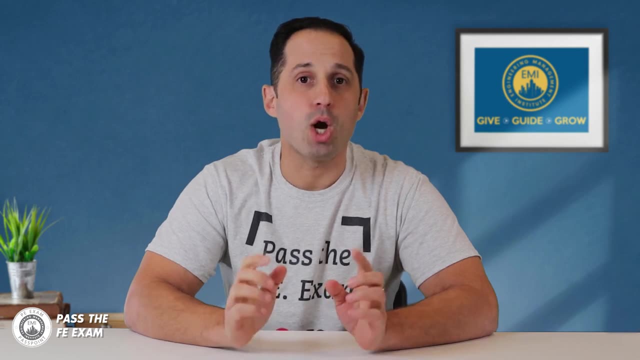 process of designing new structures. Now, after performing a preliminary design, the designer will have the opportunity to choose which forces to use in the next step. The design is then designed and created based on the analysis and the configuration of elements of a structure. 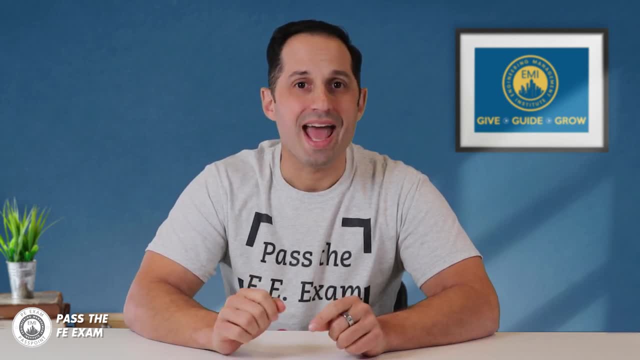 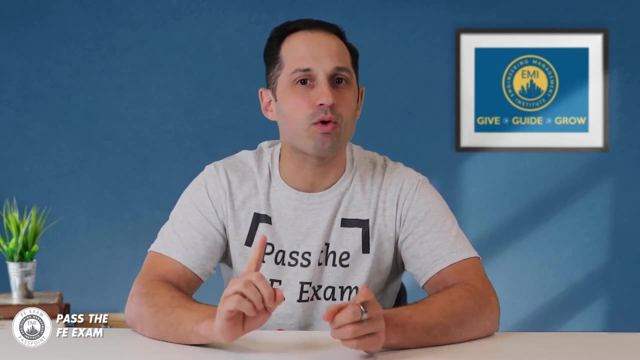 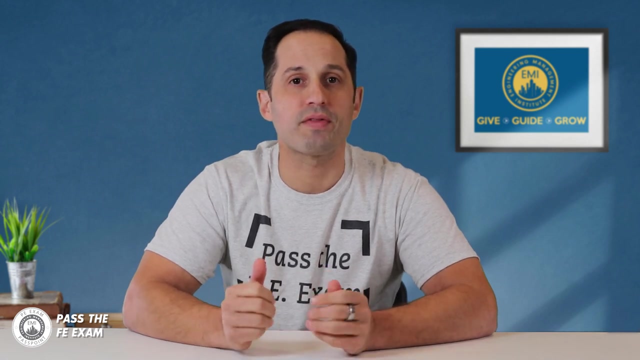 but only until an analysis is performed can the forces in those elements be known. This is really exciting stuff. After performing an analysis, the element forces are then known and the elements can be designed or their configuration can be chosen more precisely. The process iterates between analysis and design. 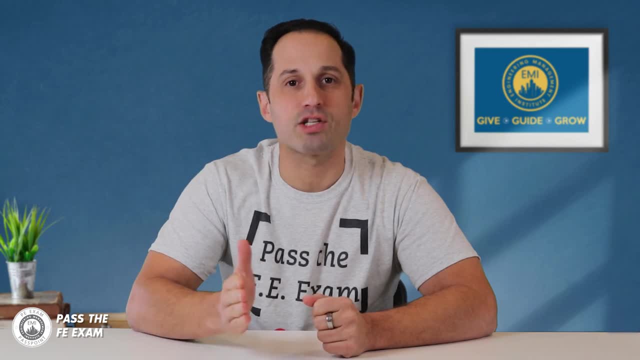 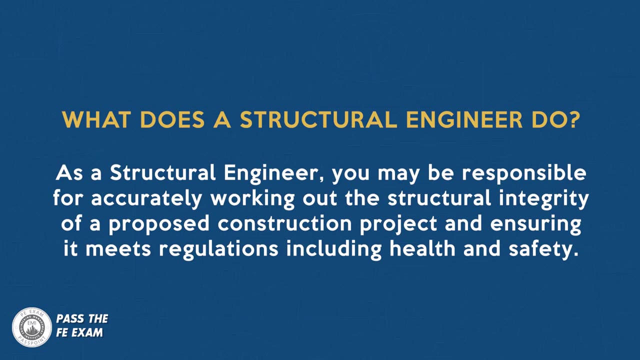 do as a structural engineer and what your tasks may look like on a daily basis. so let's take a look. as a structural engineer, you may be responsible for accurately working out the structural integrity of a proposed construction project and ensuring it meets regulations, including, of course, health. 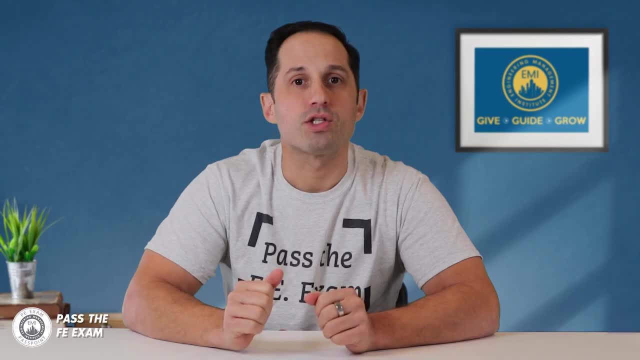 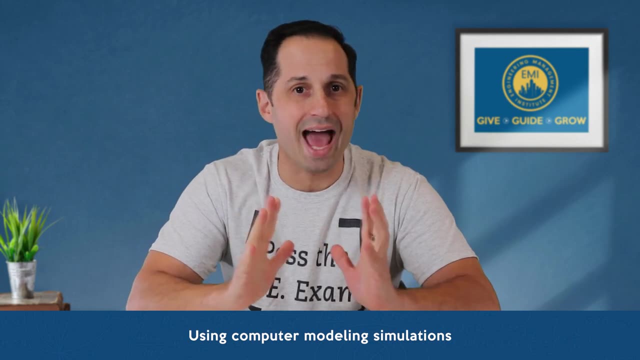 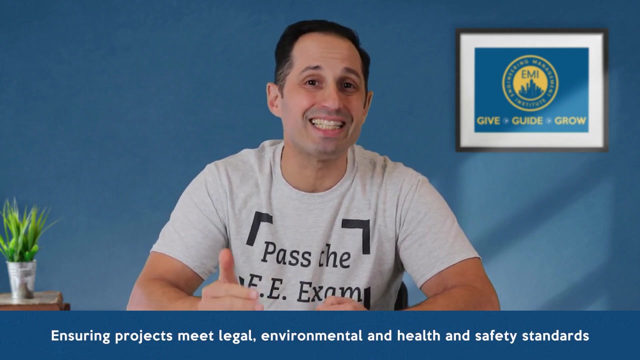 and safety, again a very challenging profession. some common tasks may include: using computer modeling simulations to predict how structures will act under varying conditions, for example high winds, flooding- which we've had a lot of- or earth tremors. calculating loads and stresses on structural foundations, beams and walls. ensuring projects meet legal environmental. 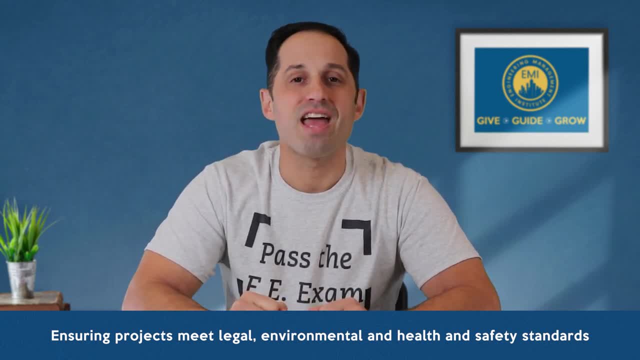 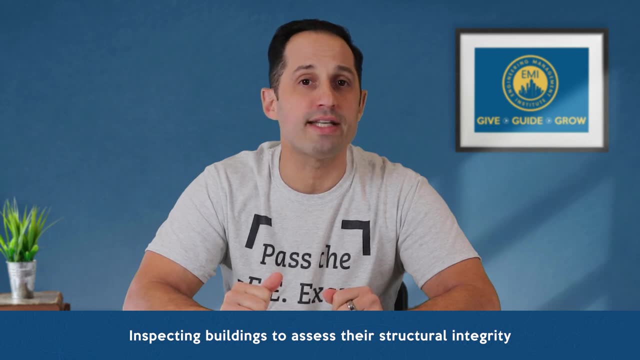 and health and safety standards. so it's not just calculations. advising on suitable materials for a build or a building, inspecting buildings to assess their structural integrity and structural integrity. another really really important task- advising on building repairs or even demolition, preparing bids for tender, working with designers to develop construction. 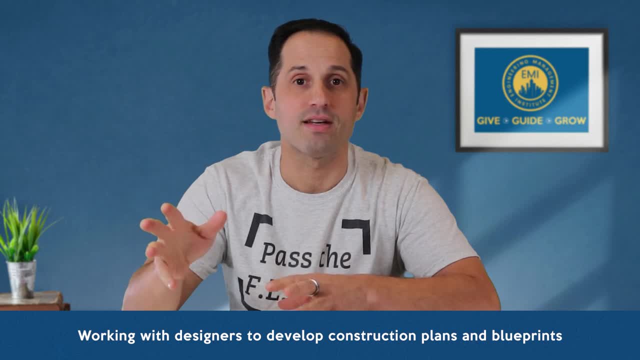 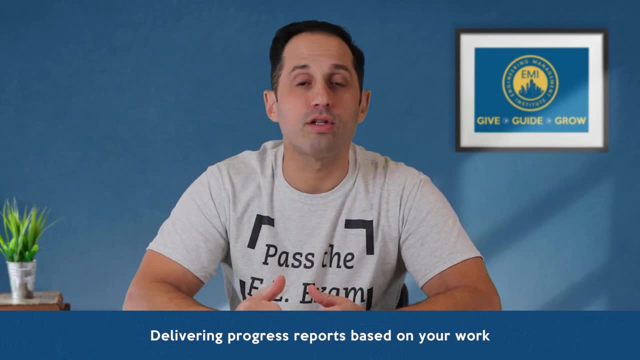 plans and blueprints so that someone can take your ideas and build them, or someone else's ideas and build them, improving a structure's energy efficiency. you can also get into energy delivering progress reports based on your work, analyzing building behavior over time, assisting with renovation or restoring heritage buildings to extend their lifespan, and working at a client's business on. 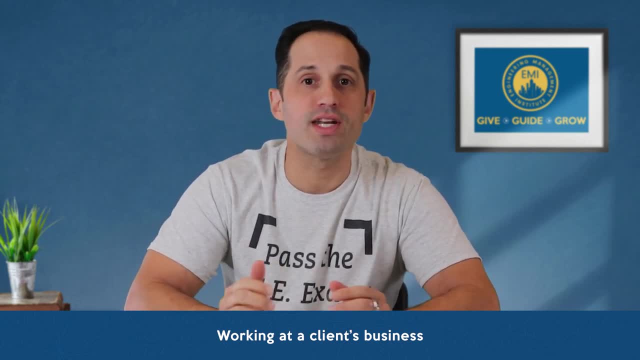 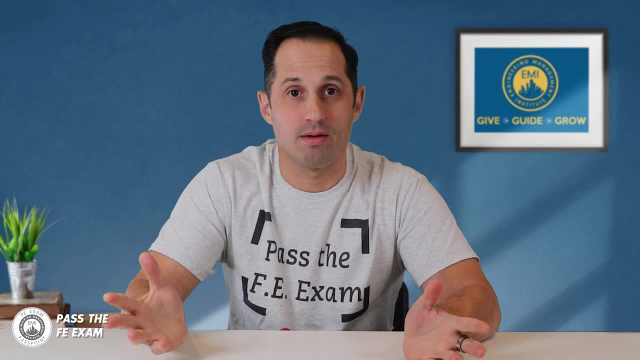 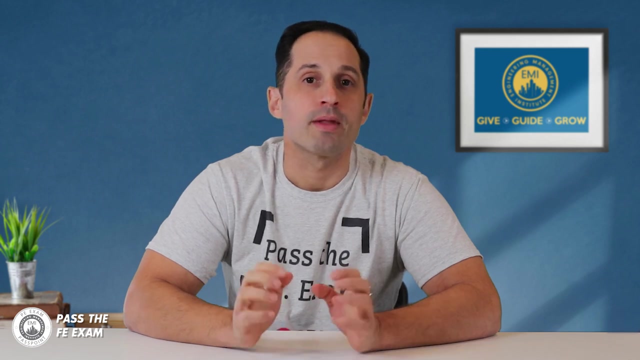 a construction site, in an office outdoors, or even in a noisy, dusty and crammed condition. essentially, as a structural engineer, you could work anywhere, both inside or out in the field. now some additional skills which may benefit anyone looking to become a structural engineer might include knowledge of engineering, science, math and technology. knowledge of 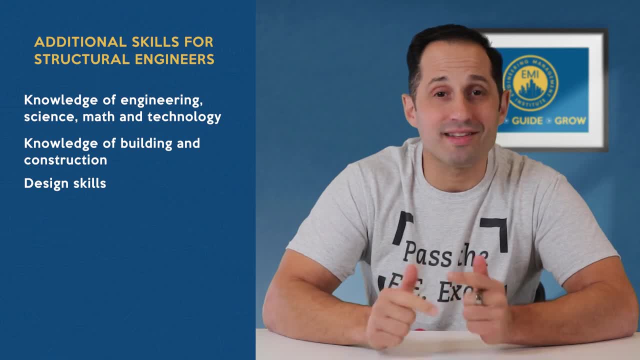 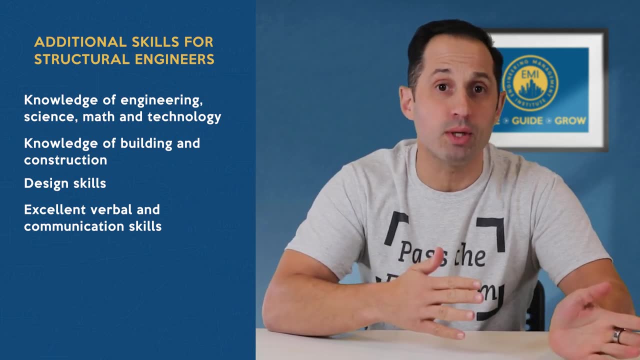 building and building. engineering and building. engineering and building. engineering and building, building and construction. design skills. You're gonna do a lot of designing as a structural engineer. Excellent verbal and communication skills. How are you gonna explain what you designed to someone who has to build it? 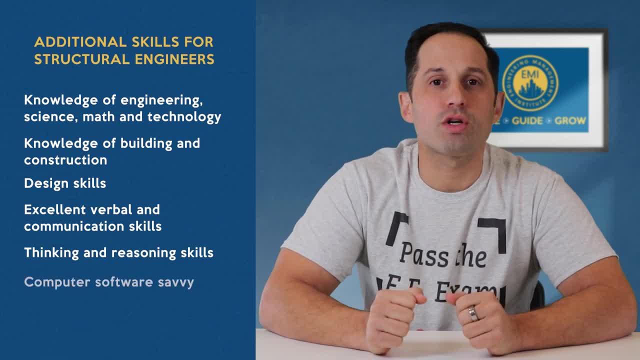 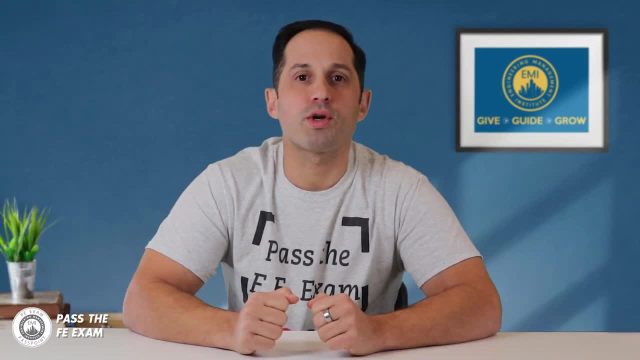 Thinking and reasoning skills and the ability to use a computer software that might help you with the structural modeling, and there are a lot of them out there. Lastly, if you were wondering how much you will get paid once you qualify as a structural engineer, 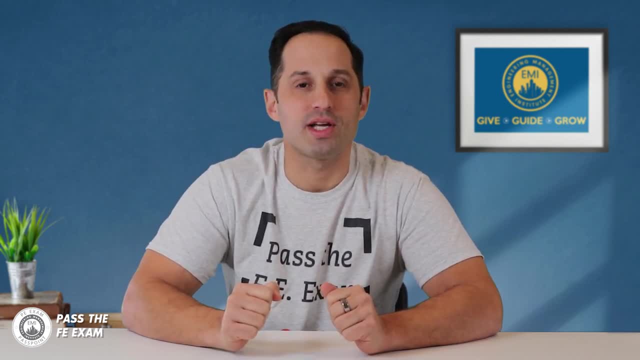 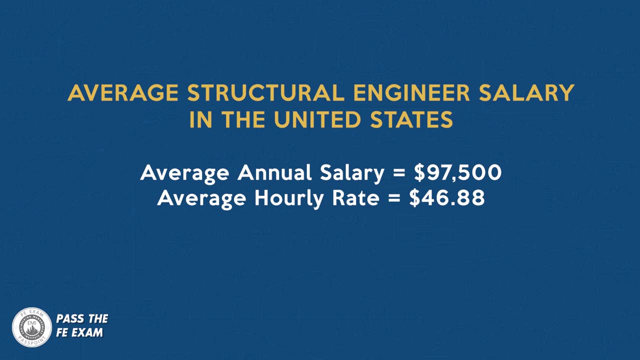 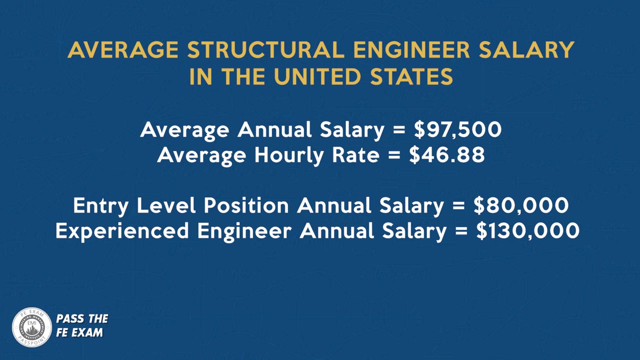 and I'm sure you are. the average structural engineering salary in the United States is $97,500 per year or $46.88 per hour. Entry-level positions start at about $80,000 per year, while an experienced structural engineer can make approximately $130,000 per year.